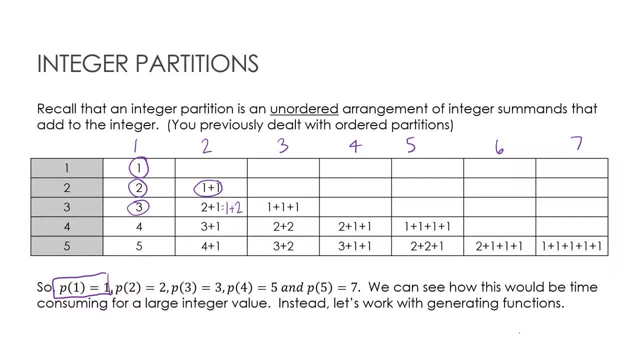 P of 3 would be 3.. P of 4 would be 5, and P of 5 would be 7.. Now if I ask you, what's P of 32?? Well, that would be much more time-consuming. 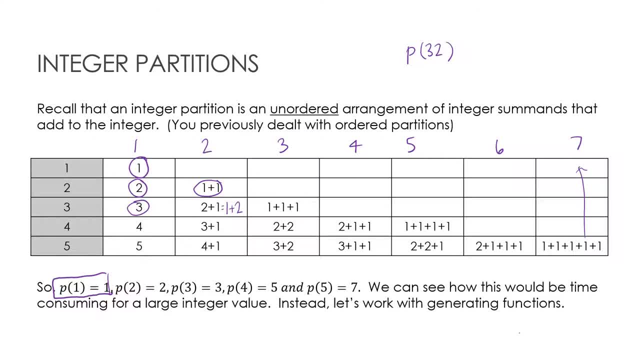 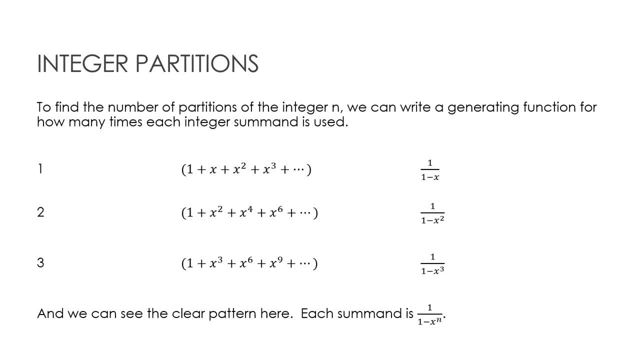 So what we want to do is look for a way to do this with generating functions. Essentially, how we do this is we look at: how many 1s would I use. So how many 1s? Well, that generating function would be that I could use 0 1s. 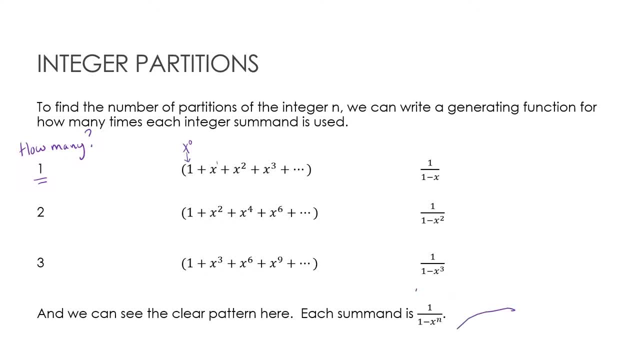 which, of course, x to the 0 is 1.. I could use 1 or 2 or 3,, etc. all the way to infinity, until whatever n is that I'm trying to solve for How many 2s? 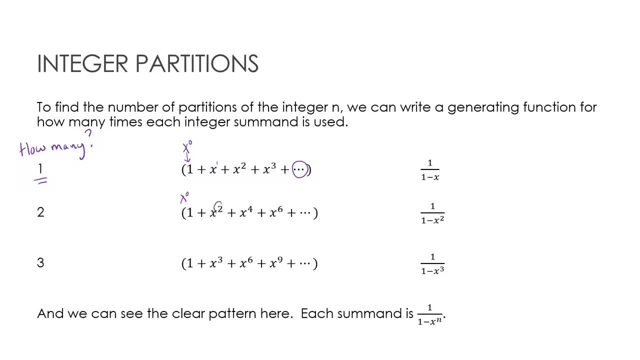 Again, I could use 0, 2s And remember I'm going to go straight to x squared here because I want my exponent to represent the value of the x squared. So I'm going to go straight to x squared here because I want my exponent to represent the value of the x squared. 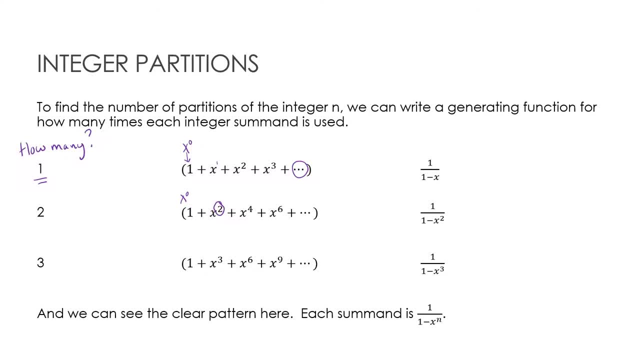 value, So I wouldn't use x to the first, even though it's 1,, 2, I'm really adding two values, So 2,, 4, 6,, etc. 3, 6, 9, or 0,, 3, 6, 9,, etc. for threes, And we can see how this pattern would. 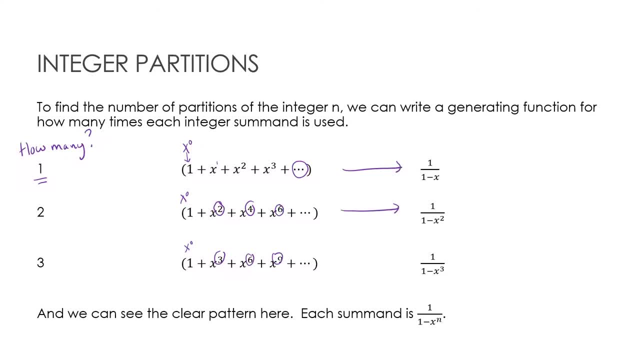 continue. Looking back at how we then wrote the each of these generating functions, this would be 1 over 1 minus x. that was just that fundamental identity from section 9.1.. If it was going by twos it was 1 over 1 minus x, squared 1 over 1 minus x to the third, etc. And you can see: 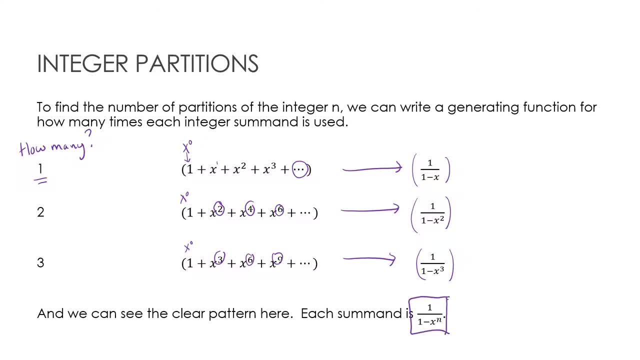 that it would be essentially all the way up to 1 over 1 minus x to the n. So whatever I'm doing, it's really just going to be 1 over 1 minus x, times 1 over 1 minus x, squared times 1 over 1 minus x to the third, etc. All the way to 1 over. 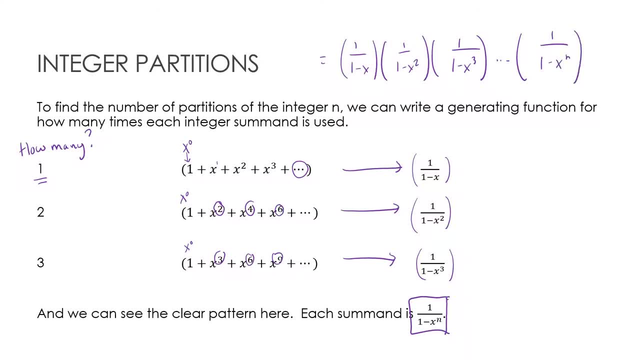 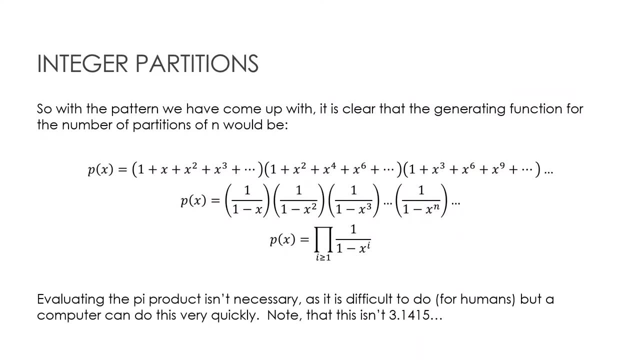 1 minus x to the n, And that's how I'm going to find the number of partitions of n. So, again, the number of partitions of n would be exactly what we just went through, which is writing all of this, and this is where I would end up Now. previously we learned summation notation: Summation notation. 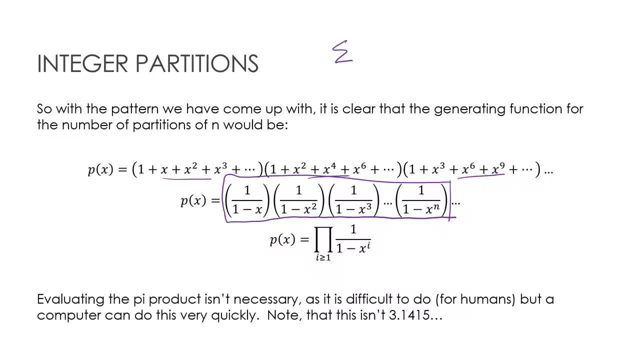 means add up whatever values that you have. So we're very familiar with summation notation. This might be a new notation for you, perhaps not. This is essentially the same thing as sigma, but this means product, So it's a pi product And essentially I'm saying: go from where x is 1 to where x is infinity. So I could. 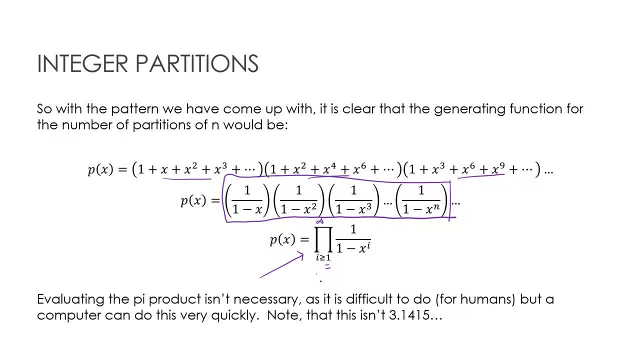 write it: i equals 1 to infinity. Or note: I just wrote: i is greater than or equal to 1, because it implies that it keeps going forever And I'm taking 1 over 1 minus x to the i, And so essentially, 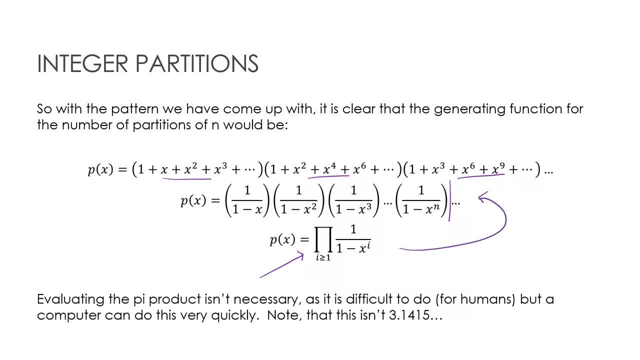 that's saying the same thing as this. It's saying: take the product of all of those values until you get to n Again, it doesn't make sense for us as humans to calculate the pi product just like. I would. let you keep your answers in. you know your binomial coefficient notation previously. All I want you to do 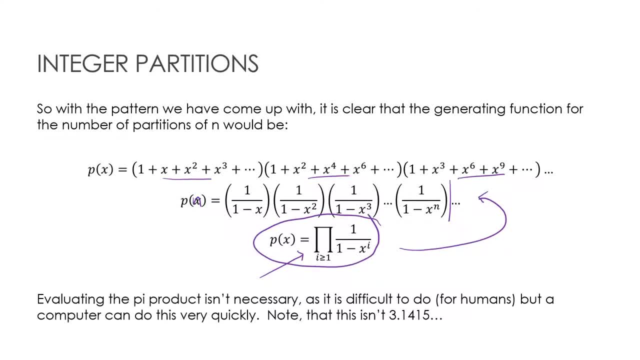 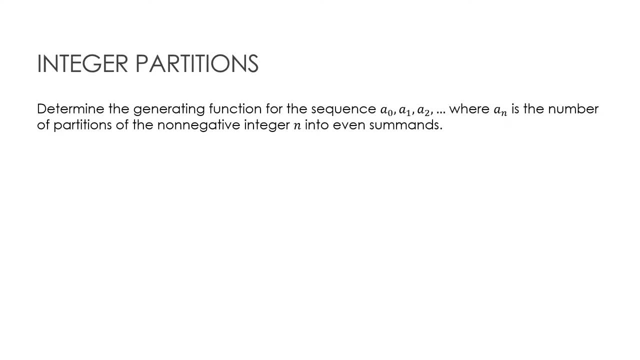 is come up with the pi product because computers can calculate that in a snap. Looking at the same concept, I wanted to determine a generating function for a sequence where a, n is the number of partitions of non-negative integer into even summands, which meaning I'm looking for only even values. Well, we can tell that instead of 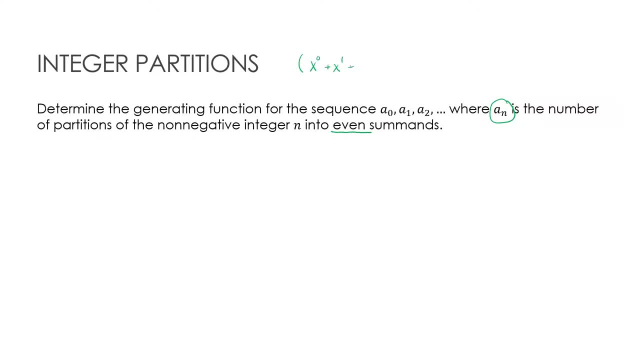 x, 0,, x1,, x2, I would be going straight to x2,, x4,, dot, dot, dot, And then if I went by 4s, and then if I went by 6s or 8s or tens, et cetera again. 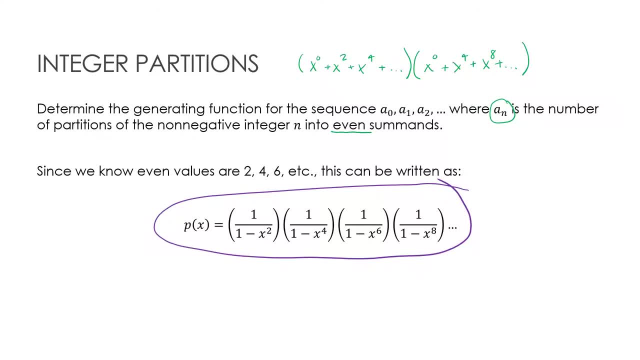 I'm looking at something that looks like this, so I'm only looking at the even values. again, how would I write that with my PI product notation? again, you can either write it this way with the PI product, or I could have used the same that I. 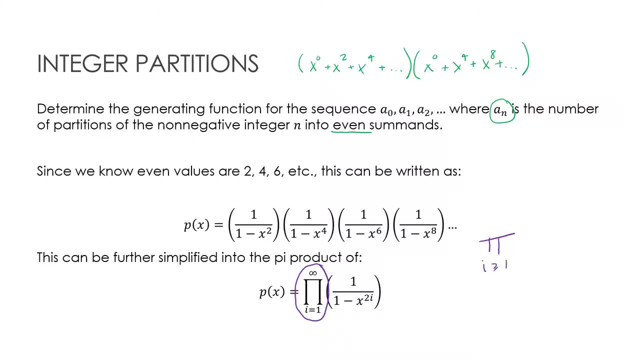 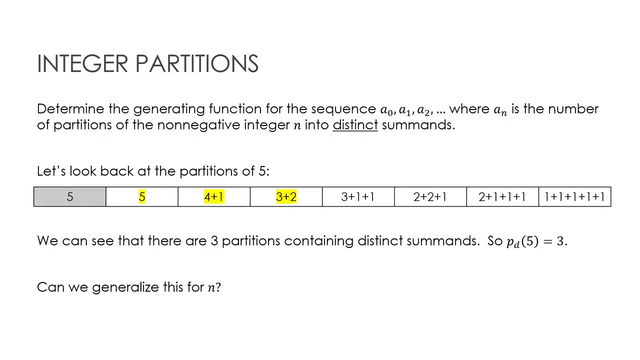 used before I is greater than or equal to 1, but notice, what I've done here is: I basically said it's going to be even because I'm going to take I times 2, so that's only going to give me even values here. let's change it up yet again. now. this one is asking about distinct summons, which means 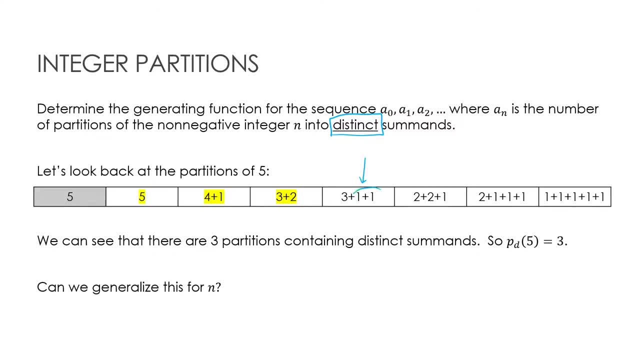 I don't want to have something like this, where I've used one more than once, or two more than once, or one more than once or one more than once. so, looking back at the partitions of five, and even though p5 was seven, if I'm looking at the distinct partitions, p sub d, I'm telling us that 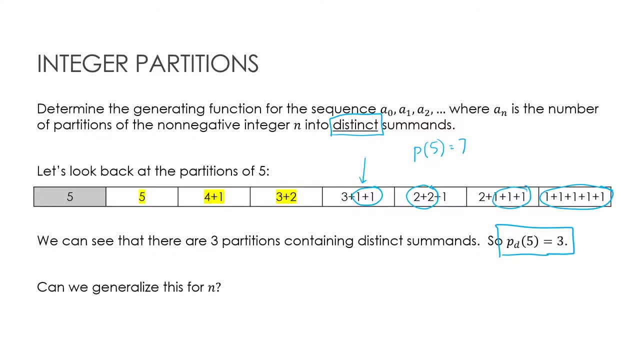 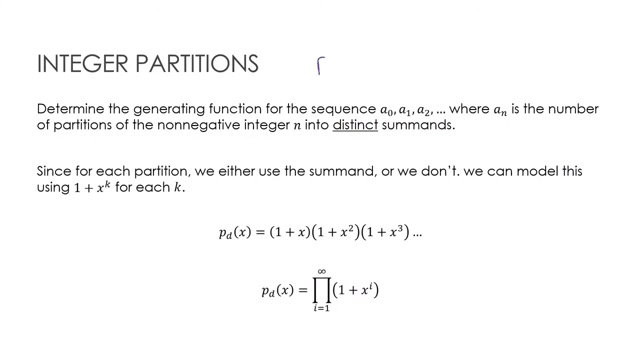 it's distinct of five. there are only three of them, five, four plus one and three plus two. so my question now is: can I generalize this for n? so can I write something where p sub d of n is equal to something general? can we generalize that for p? d of n? or saying: can we generalize we're looking at? 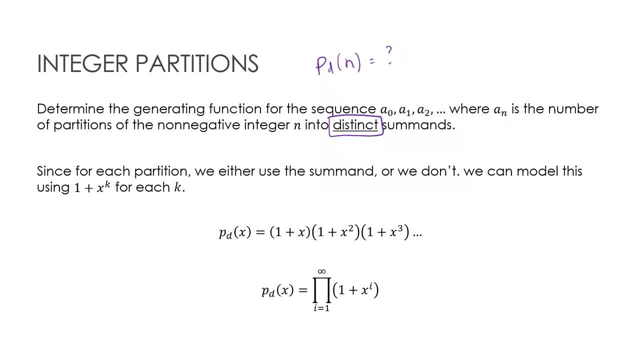 distinct summons. so if we think about distinct, we're basically saying: I'm going to use a one or I'm going to not use a one. I'm going to use a two, which would add two to our sum, or I'm not going to use a two. I'm going to use a three or I'm not going to use a three. so we get the idea that that 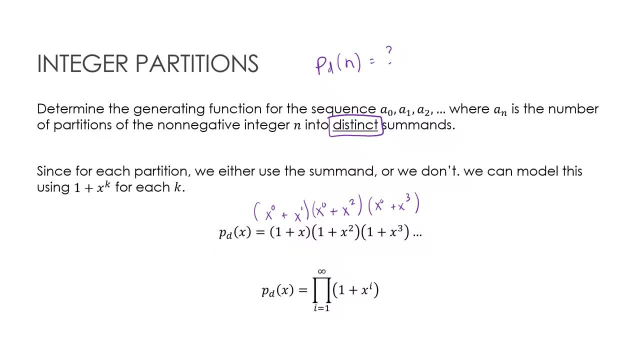 pattern would continue to write it as a pi product. I'm going to write it as the pi product of one plus x to the i. so again, I'm multiplying one plus x to the first, one plus x to the second, one plus x cubed, et cetera, et cetera, all the way up to whatever value I determined that I'm trying to solve for. 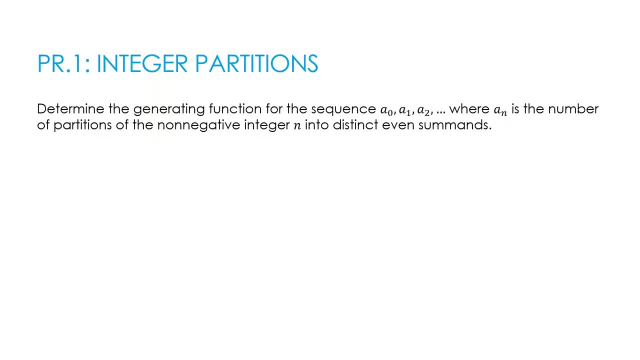 here's an integer partitions question for you to try on your own. I'm asking for the generating function again. write it as a pi product. don't evaluate for the sequence where a sub n is the number of partitions of non-negative integer n into distinct, even summons. when you are ready, 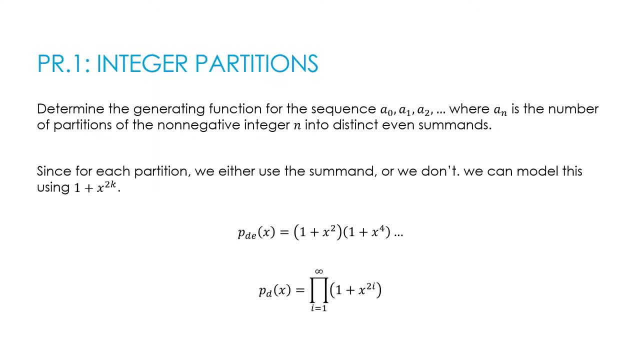 press play to see how you did again. so we're looking for distinct and we're looking for even. so. we're kind of putting two things together that we've already sort of talked about again, for each partition, we're either going to use the summoned or we're not, which we can model using one plus x to the 2k. so why did I choose 2k? 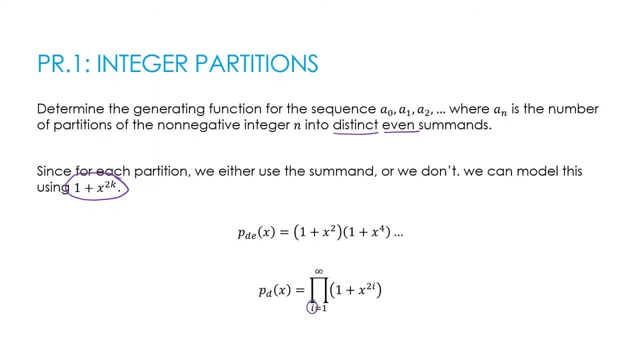 or 2i or whatever letter I choose. again here I used I. so in my final answer I used I. why did I use two? because we're looking for even summons only so I'm looking for x, squared x to the fourth, again not using six or using six. 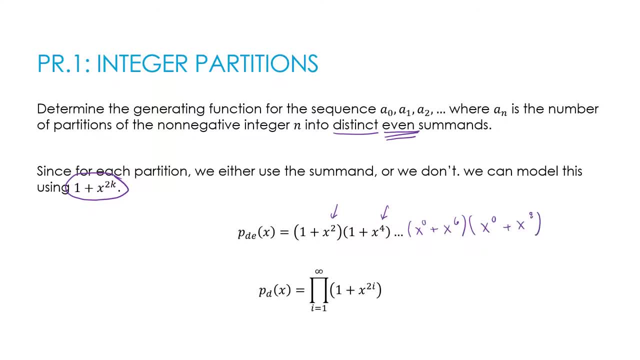 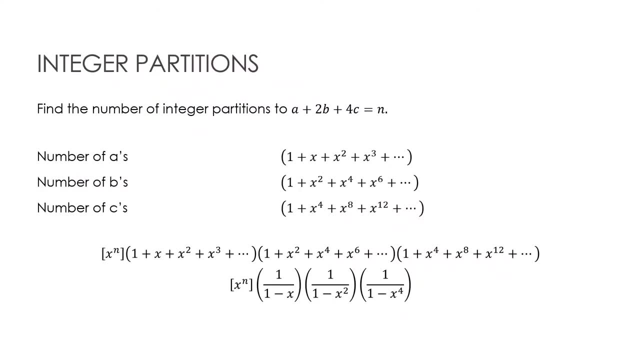 not using eight, or using eight, et cetera, et cetera, et cetera. that is how we're going to write that Pi product. here's a very common application of integer partitions. let's say, I'm trying to find the number of integer partitions of 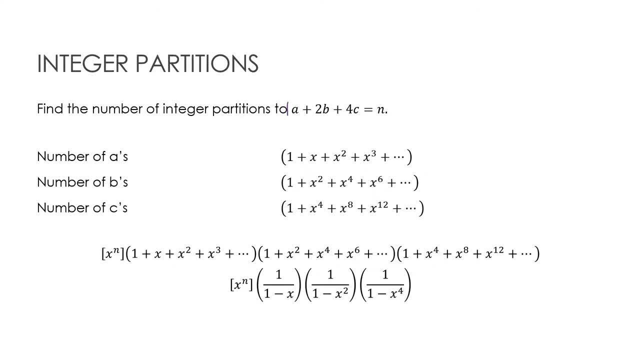 For a plus 2b plus 4c, and again it would be 1a, 2b, 4c equals some number. So my question is: how many a's will I use? Well, a's go up by 1,. so notice, I'm just having my exponent increase by 1,. 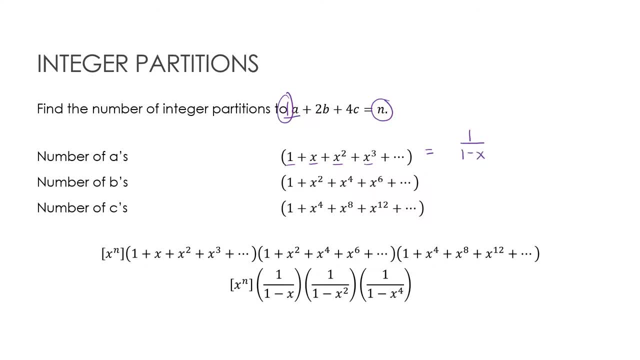 which I can write as 1 over 1 minus x For b's. that will increase by 2.. Remember, I can write this as 1 over 1 minus x squared For c's. each time it will increase by 4, so that's 1 over 1 minus x to the 4th. 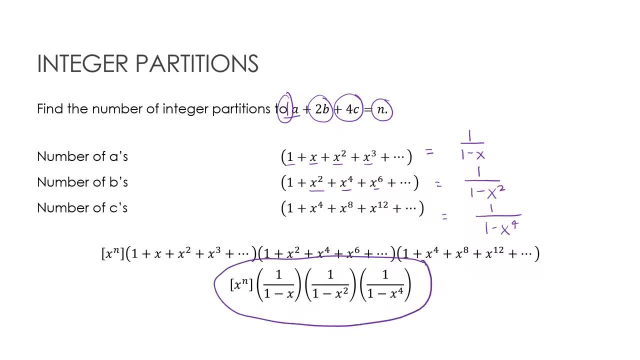 So my solution is: whatever n happens to be of this product. So here's another to look at: 27a plus 42b equals 192.. What's the number of integer partitions? Well, I know that I'm looking. I'm looking for x to the 192, which means the coefficient for when x is equal to 192.. 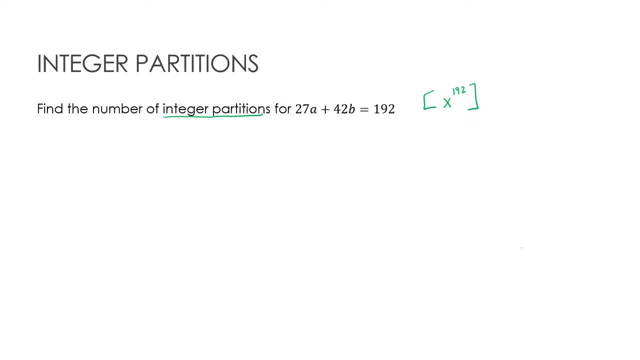 I'm sorry. when x is to the 192nd power, How would I write this? Well, I can write this out as: x to the 0 plus x to the 27 plus x to the 54, etc. Oops, Plus, dot, dot dot. 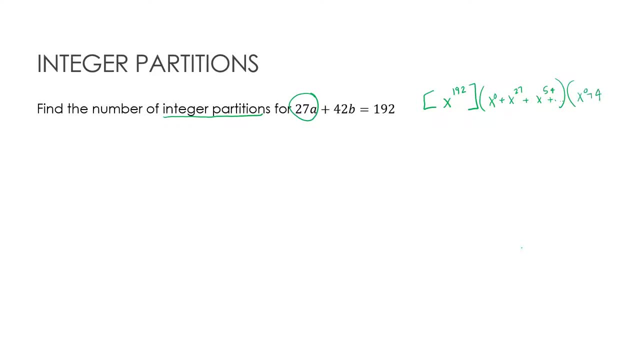 For 42,. it would be x to the 0,, x to the 42,, x to the 84,. dot, dot dot. But really I don't care about that line of work. What I really want is: how am I going to write this? 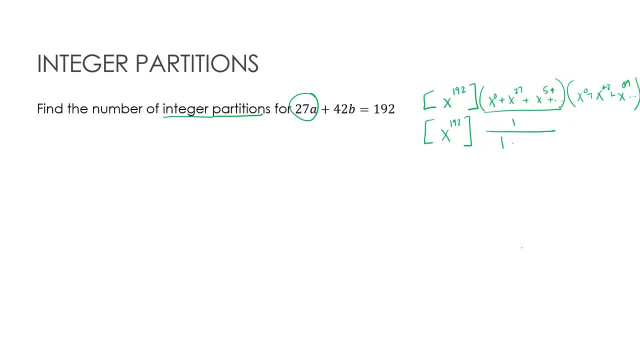 Well, that's 1 over 1 minus x to the 27. And this is 1 over 1 minus x, And this is 1 over 1 minus x to the 42. And again, that's all I have to do. 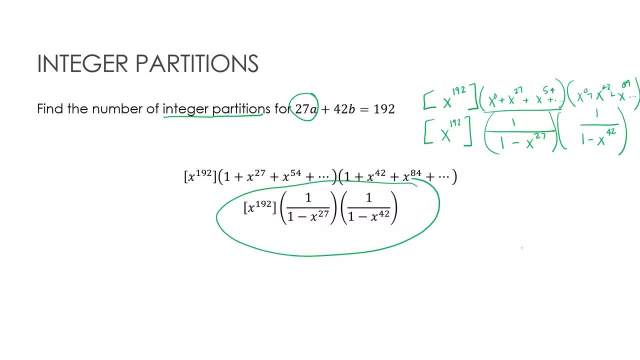 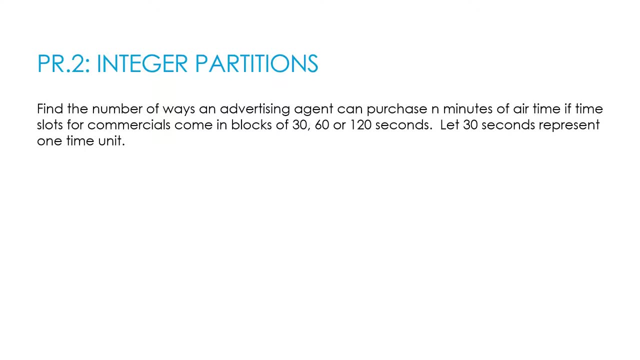 I don't have to work anything out, I just have to write it symbolically. Here's a first question for you to try on your own. Again, I'm looking for in this case the number of ways an advertising agent can purchase. 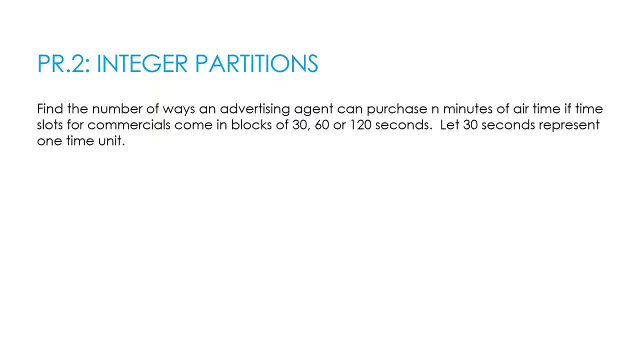 n minutes of airtime. if time slots for commercials come in blocks of 30,, 60, or 120 seconds And we're going to assume that one unit of time is 30 seconds, Try this question When you are ready. press play to see how you did. 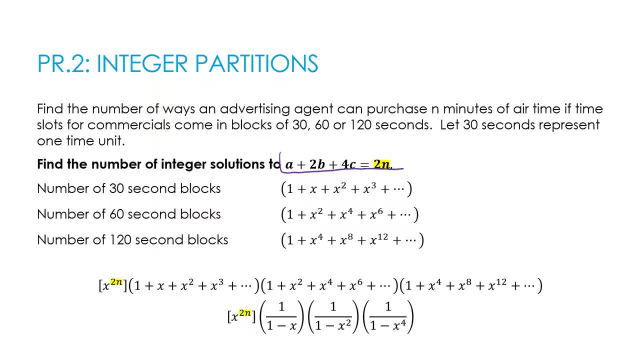 So where I would start is I would write this equation. So let's talk about this equation first. If 30 seconds is one unit of time, then if I let A represent each 30-second slot, then it would just be 1A, because that's just one unit of time. 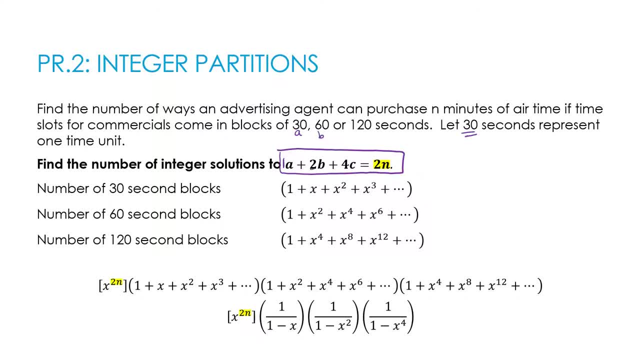 If B is 60-second slots, obviously that's two units of time, And if C is 120-second slots, that's four units of time. The question is then: why is this 2n, if I'm looking for n minutes? 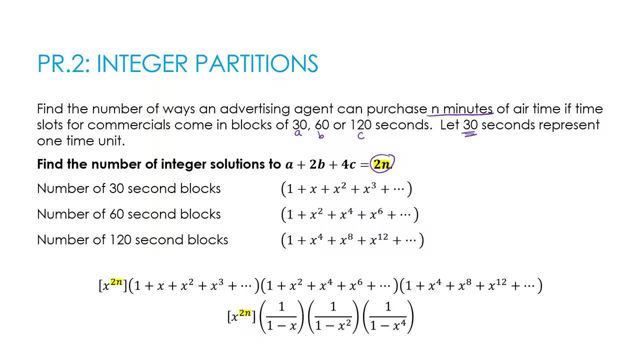 Well, we're looking at n minutes, but this is 30 seconds, And so obviously I need to take 2 times n to get the number of minutes, since there are obviously 60 seconds in a minute. So that is my initial equation. 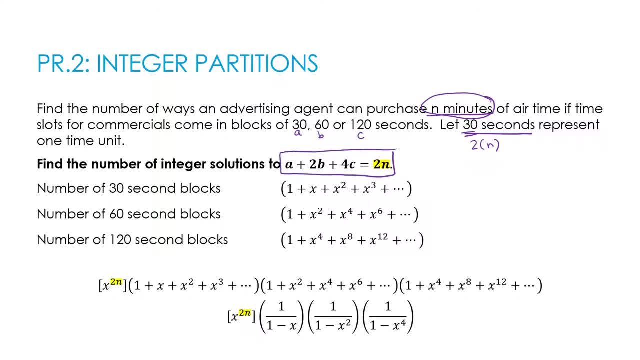 If you weren't able to come up with a number, then you wouldn't be able to come up with a number. If you weren't able to come up with a number, then you wouldn't be able to come up with a number. If you didn't come up with that equation, you weren't able to finish this question, and that's okay. 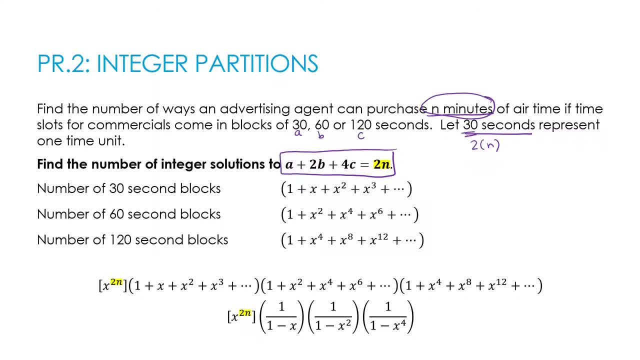 But remember this one, because the last practice will be a continuation or an alteration of this question. So again, the number of 30-second blocks: 0, 1,, 2, 3, etc. The number of 60-second blocks, remember, I'm only going to be using those, even exponents. 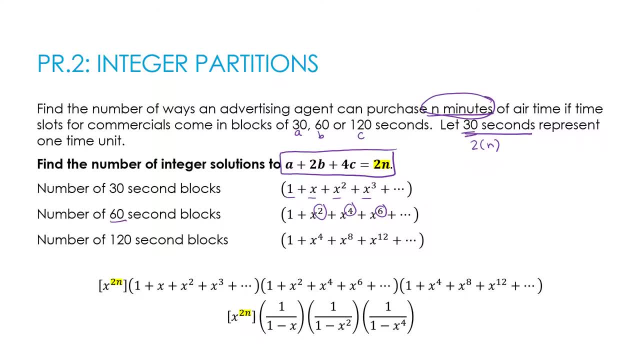 because that's going to give me two units of time, or four or six, etc. For 120, I'm going to be going by fours. And then again, because my solution to the equation is 2n, then I'm looking for the coefficient of x to the 2n. 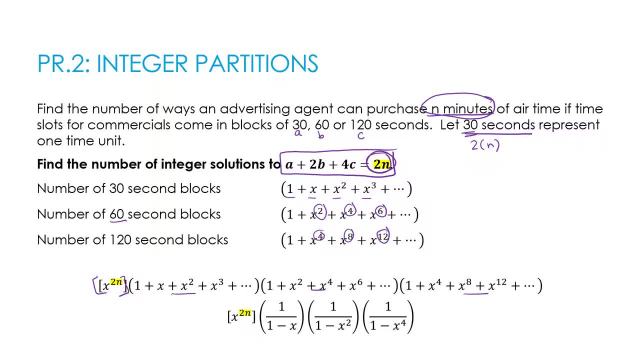 I'm taking each of these and just rewriting them. This is 1 over 1 minus x. This is because I'm going by twos- 1 over 1 minus x squared, And then again because I'm going by fours- 1 over 1 minus x- to the fourth. 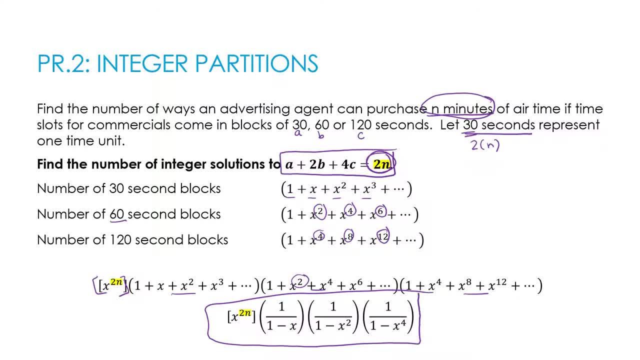 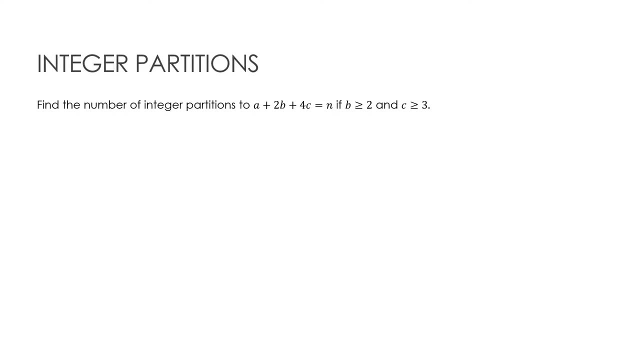 So here is my final solution. It seems so easy Once you go through it. but again, keep this equation in mind, as we're going to use it again in just a moment when we try practice three. One last question to try together, before I have you do a similar question on your own. 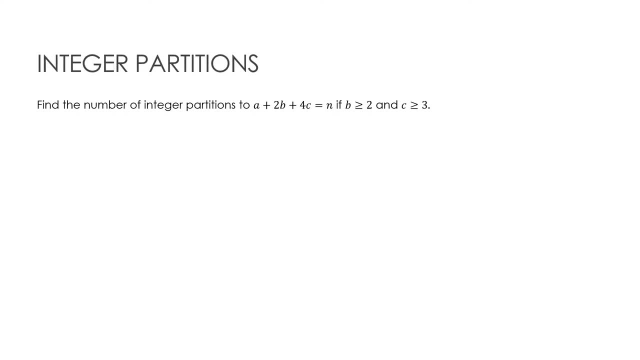 Let's take a look at what happens when I add some additional restrictions. So this should look familiar to us. where we have a plus 2b, plus 4c is equal to n. And now I'm saying: but hey, b has to be. 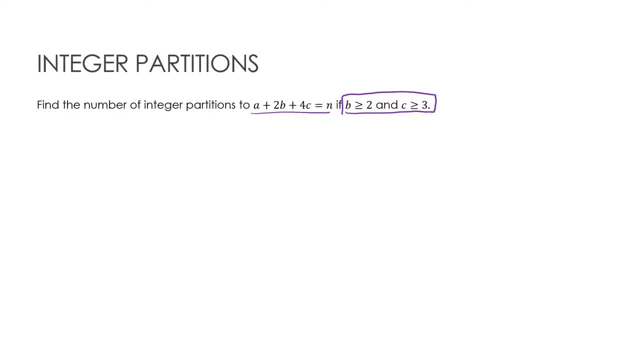 greater than or equal to two, and c has to be greater than or equal to three. So let's take a look at each one of these. now for the number of A's, That one's very straightforward. I didn't change anything. The coefficient is still one. 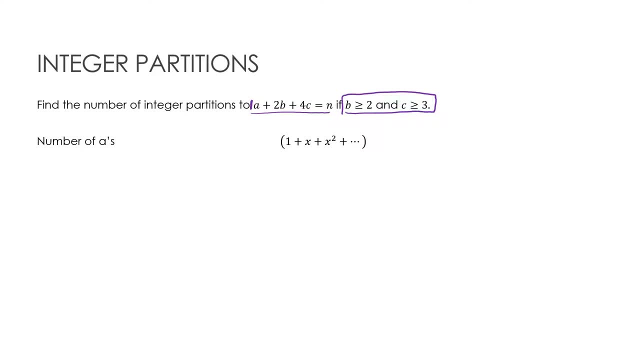 So it's 0123,, etc. For B. remember previously for B I had used x0,, x2,, x4,, x6, etc. I had used x0,, x2,, x4,, x6, etc. 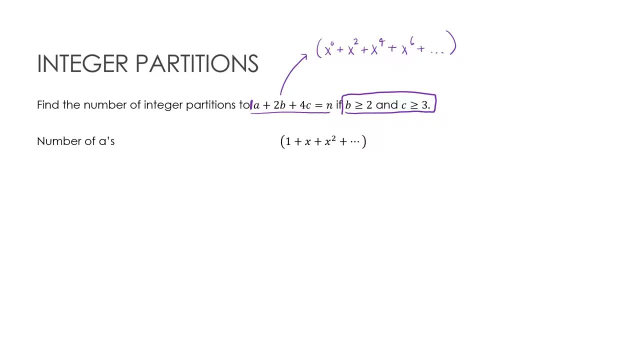 I had used x0,, x2,, x4,, x6, etc. Because I was going by twos. Now I'm saying b has to be greater than or equal to two, which means if I plugged a two in over here, 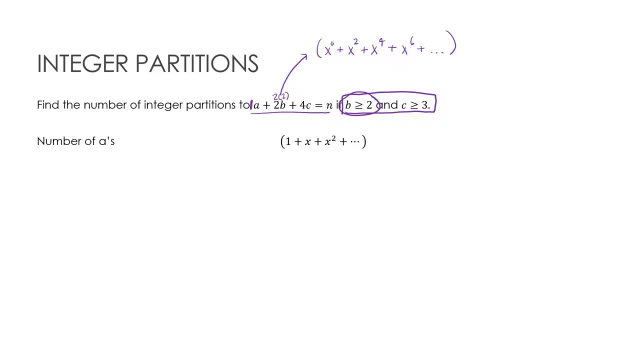 that's actually four is my very first value that I could use. So really I'm looking at x to the fourth plus x to the six, plus, etc, etc, etc. So that's for the number of B's. Similarly for C. previously I had x to the zero, x to the two, etc. etc. 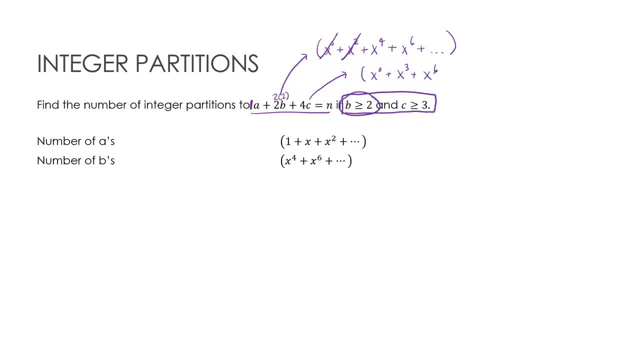 So that's for the number of B's. Similarly for C. previously I had x to the zero, x to the two, etc. etc. x cubed, x to the sixth, x to the ninth, da, da, da. Now I'm saying, oops, I'd better keep going just a little bit. 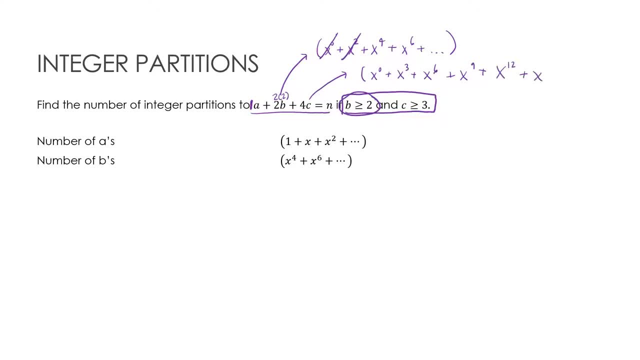 x to the twelfth, x to the fifteenth, da, da, da. And now say: three times four is twelve. So twelve is the first one. so I have x to the twelfth, x to the fifteenth, etc. on forever. 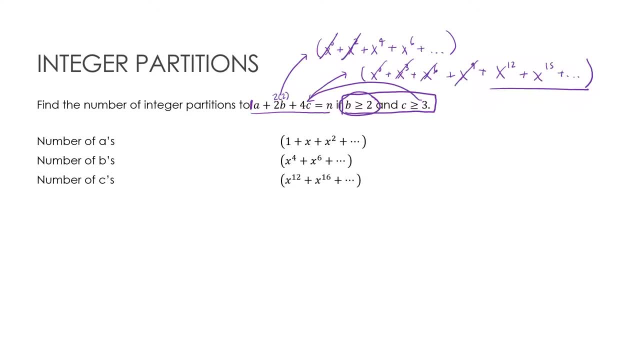 For the number of C's. From here. what I want to do is kind of put this all together, but keep in mind that, while I can still rewrite this as 1 over 1 minus x, this is now going to be an x to the 4th taken out. 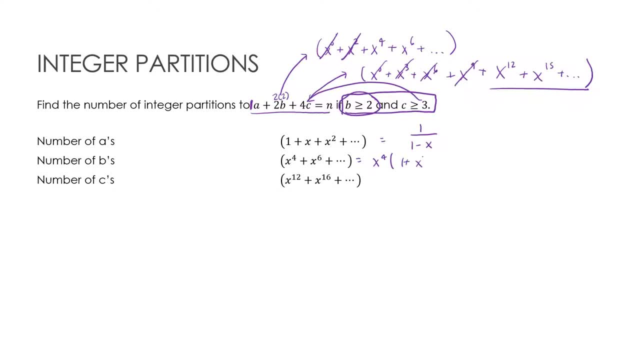 and then I will have 1 plus x squared plus x to the 4th, which can be written as x to the 4th over 1 minus x squared, So the x to the 4th that I have factored out. 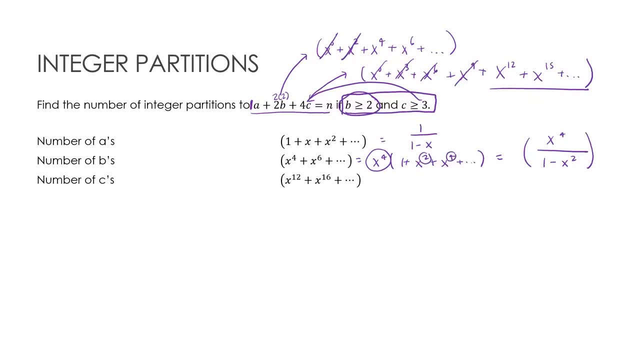 and the 1 minus x squared because I'm increasing by 2.. And same concept here I'm going to take out x to the 12th and then I would be going up by 4s, And so to simplify that that would be x to the 12th over 1 minus x to the 4th. 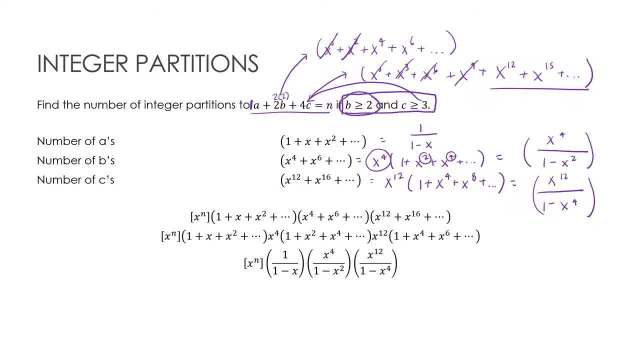 The next step, then, would be to essentially write it as a generating function. So I'm trying to find x to the n, because that's the solution to my equation, And what do you suppose is going to come next? Well, I've got 16 x's. 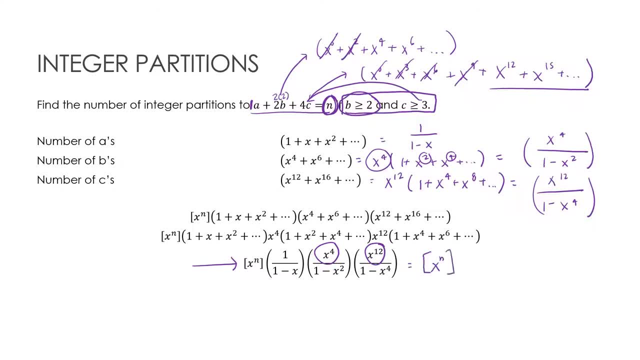 So really, this is x to the n, And then I've got x to the 16th times: 1 over 1 minus x, 1 over 1 minus x squared, 1 over 1 minus x to the 4th. 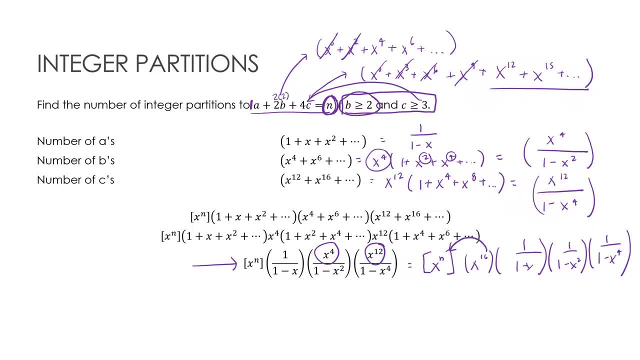 Just as we did before, I'm going to sort of smush those two together and say let's go ahead and shift it back. So now I'm looking for x to the n minus 16 of all of this, because I've shifted it by 16.. 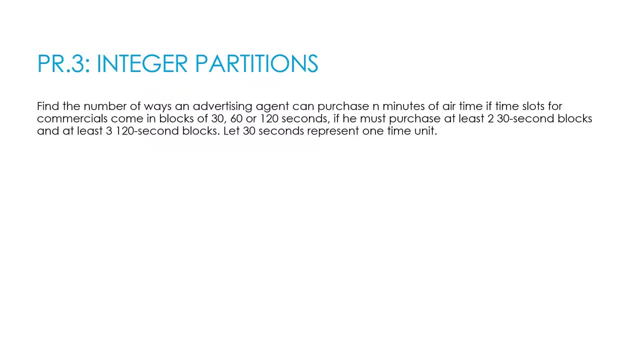 Here is your last practice, tied very closely to practice 2. that we did already. The only thing I've changed now is I've given you some restrictions. You must purchase at least two 30-second blocks and at least three 120-second blocks. 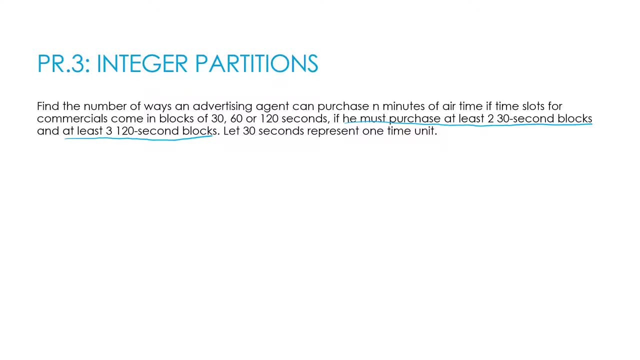 Everything else remains the same. So see if you can incorporate what we just talked about, with the further restrictions, into this question. When you're ready, press play to see how you did So. what hasn't changed? This guy hasn't changed. That's the same equation we came up with before. 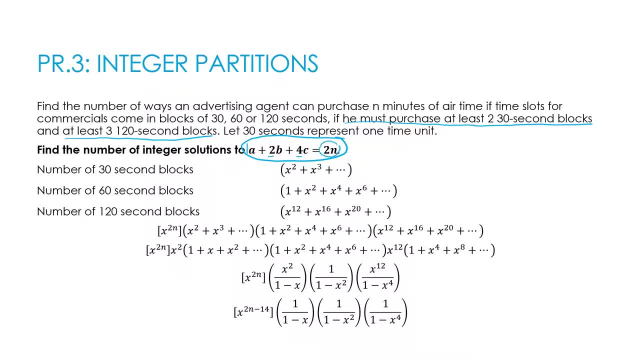 This is one block, two blocks, four blocks. We said it had to be 2n because n was number of minutes of airtime, and so we would need two 30-second units to create one minute. So that part did not change. 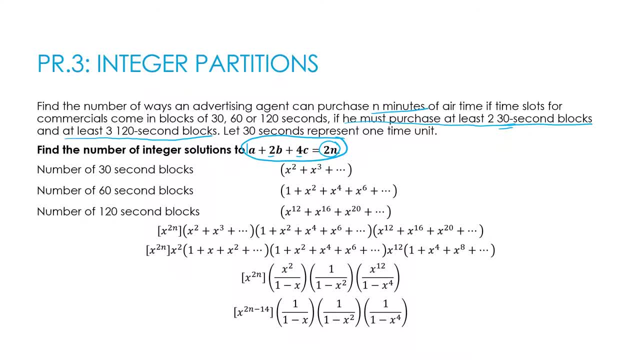 Number of 30-second blocks. it says he must purchase at least two 30-second blocks. So notice, this guy did change. That is now x, starting with x squared, which means again that what I would do is take out an x squared. 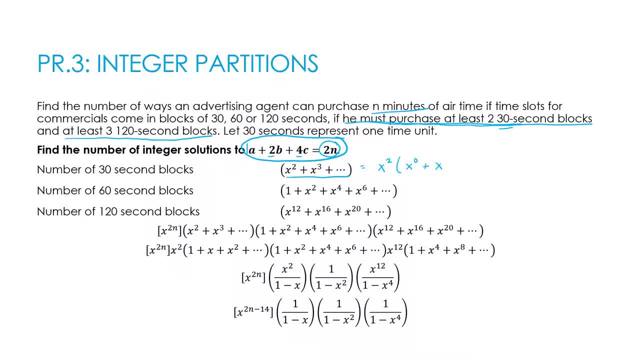 to get that x to the zero as the first value, which means I would be writing that as x squared over 1 minus x, which is where I got this value For number of 60-second blocks. this one did not change. No change at all. 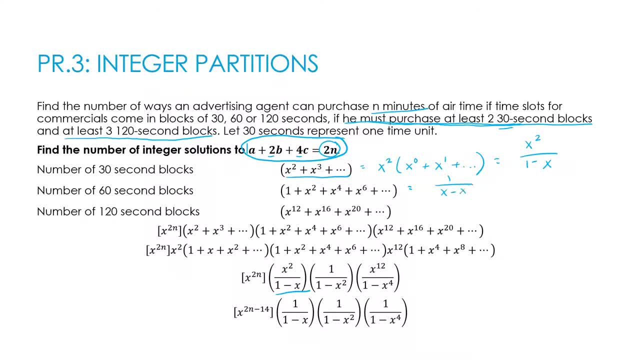 So we're looking at 1 over, 1 minus x squared- Oops, not x minus x squared, I apologize. And that's And that's this value. And then, for one 20-second blocks, I need at least three of those. 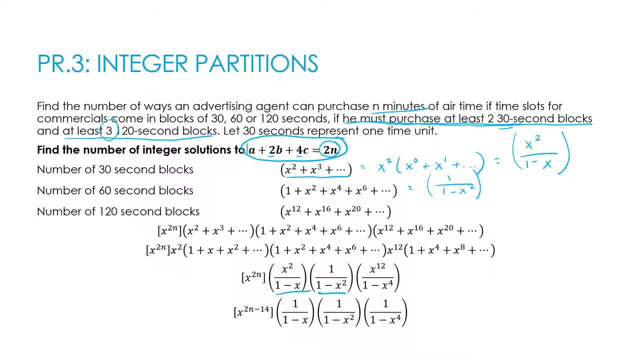 So again, I'm looking at getting rid of the first three values, which is x to the zero, x to the- because we're going by four units- and x to the eighth. So that's where I'm starting, with x to the twelfth. 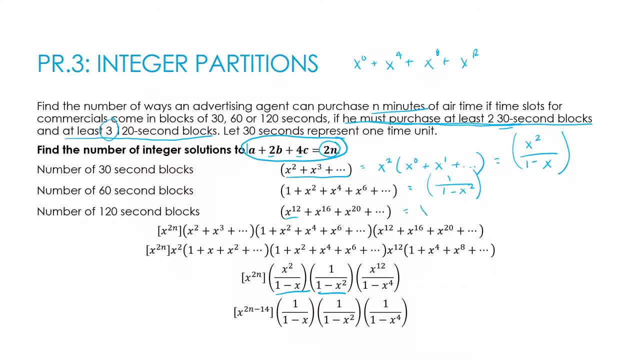 So 12,, 16,, 20,, etc. Just as I did before, I'm going to factor out in this case x to the twelfth, so that I can have x to the zero as my first term, and now I'm increasing by fours. 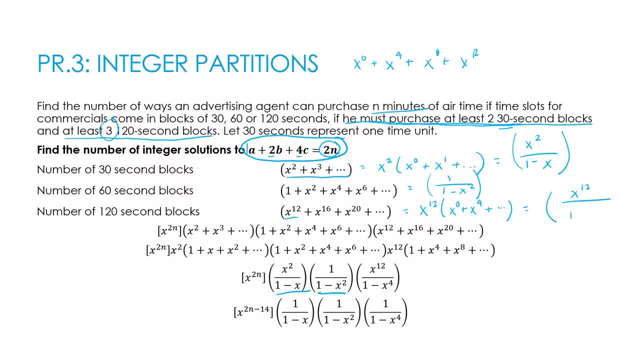 So that is rewritten as x to the twelfth over 1 minus x to the fourth. Like I did in my last example, I'm going to consolidate my x's, so this is really x to the fourteenth in front of all of this. 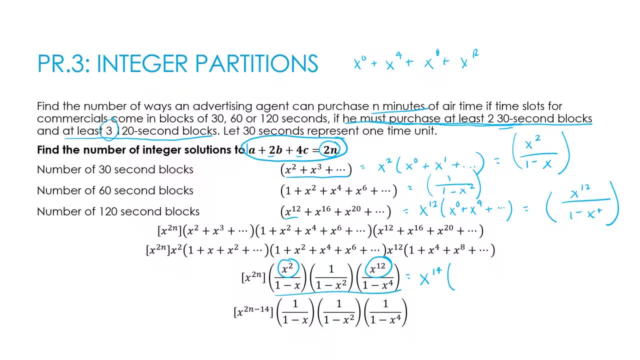 now with ones as the numerators, And so essentially I've just taken the minus 14 and basically subtracted 14 from 2n, and that is going to give me the expression that I need. 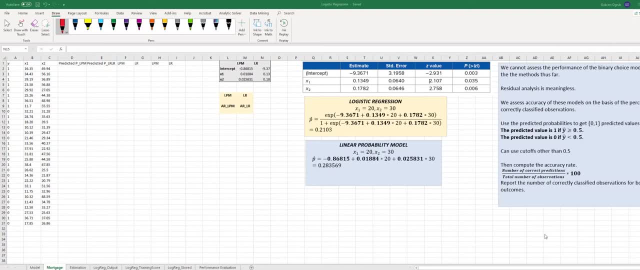 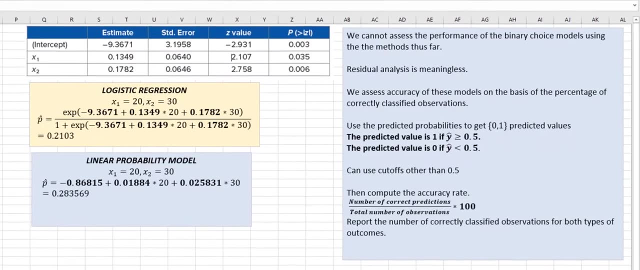 In this video we are going to talk about performance evaluation of binary choice models. There is no universal goodness of fit measure for binary choice models that can be used to assess how well the model fits the data, Unlike in the case of linear regression models. 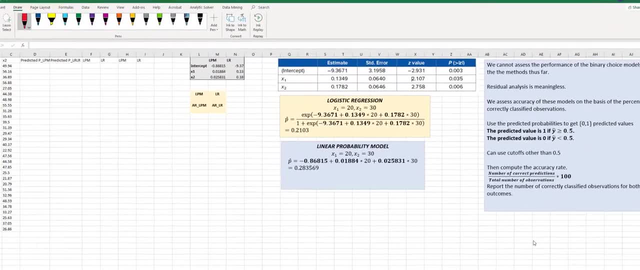 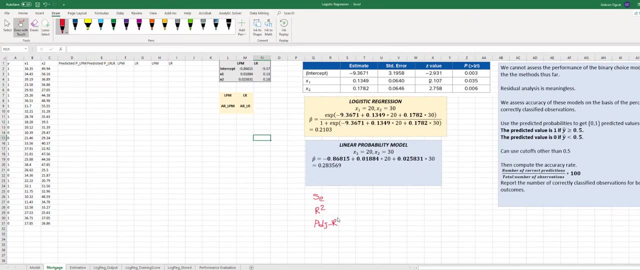 we cannot assess the performance of binary choice models based on the standard error of estimate, S e r square or adjusted r square. The residualanalysis is meaningless as well, So remember: the residual is the difference between actual data and the predicted value.